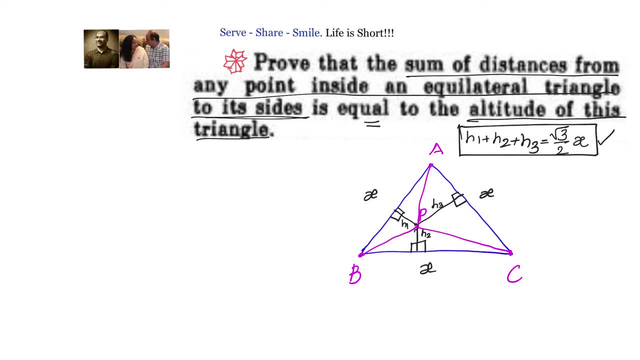 triangle APB, Then we have triangle BPC, Then we have triangle APC. We have three triangles. ABC is divided into three triangles. Now we can easily find out the area of these three triangles. So our logic is to equate the area of the triangle which we 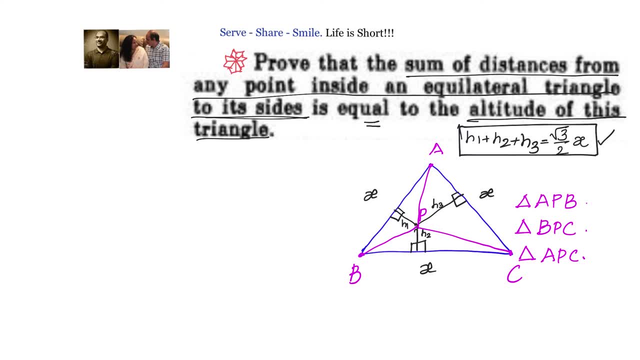 know already as root 3 by 4 into x side square to the sum of these triangles. So I will write down here: area of A B, C is equal to area of A P B plus area of B P C plus area of A P C. 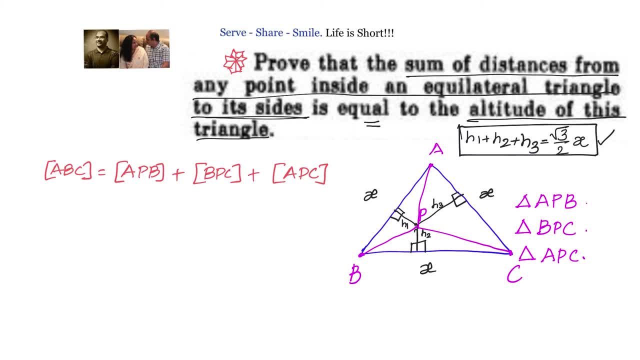 We know area of equilateral triangle. if side is x is root 3 by 4 into x. square equals to half into area of A P B is half into x, into h1.. B- P C will be half into x, into h2, plus A P C will be. 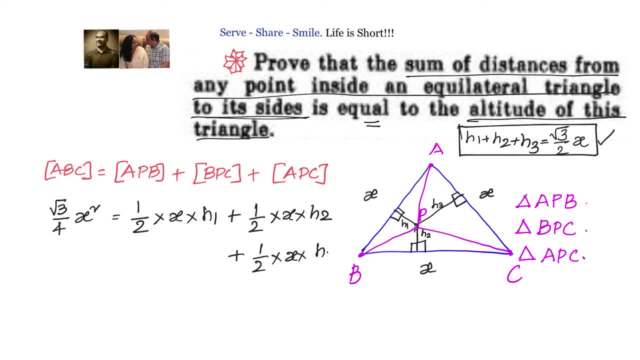 half into x, into h3.. Now let us try to simplify this. We will write down root 3 by 4 into x. square equals to half into x. we can take out: We have h1 plus h2 plus h3 left out. Let us simplify that: x will cancel one time and 2 will go two times. 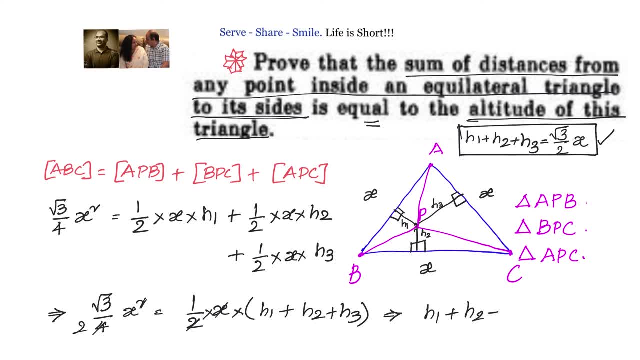 We are left out with h1 plus h3.. h2 plus h3 equals to root 3 by 2 into x. That is what we need to prove. Now, if you are not clear how the altitude of an equilateral triangle is root 3 by 2 into x. 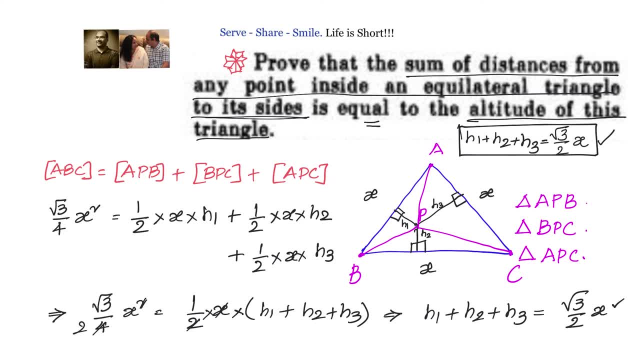 let me explain you that. Let us take the same triangle. I will take a smaller triangle since we have less space. Let us say: this is our equal Equilateral triangle of side x, x and x. If you drop a perpendicular, then by congruency we can prove that this is divided into two equal parts. 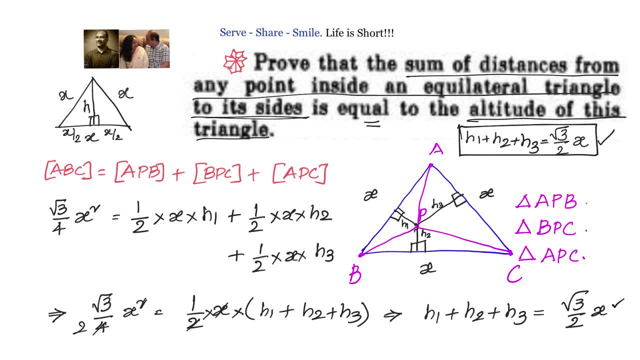 Now this is the height. Apply the Pythagoras theorem. You will have h2 equals to x2 minus x2 by 4, which is equals to 3x2 by 4.. That will give you the height. That will give you h equals to root 3x divided by 2.. 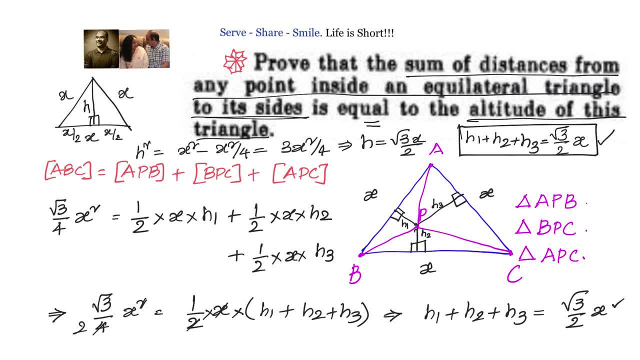 That means the altitude of an equilateral triangle is given by root 3x by 2.. And we have proven that sum of the distances from P to AB, BC, AC, sum of that is equals to root 3x by 2.. 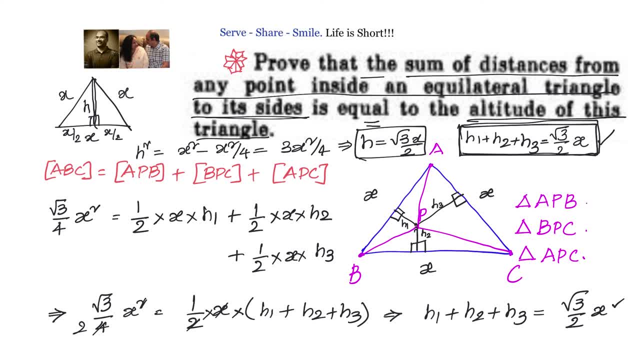 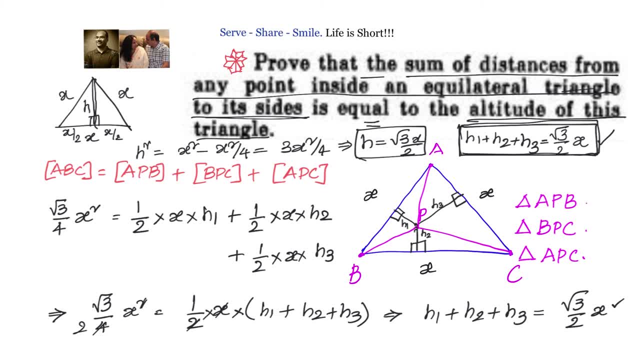 So that is how we have proven that the sum of distances from any point inside an equilateral triangle to its equal part is equal to root 3x by 2.. altitude of the triangle. Let us have a recap of this problem. Now we have been given a triangle. 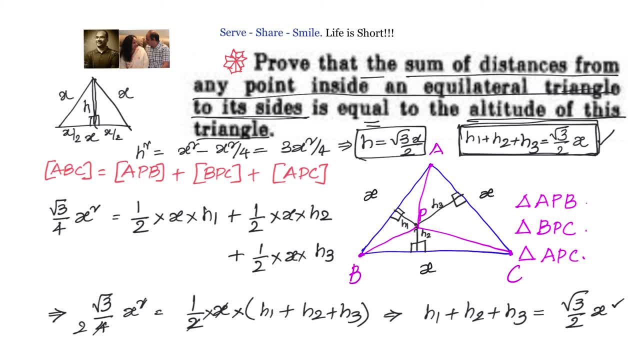 ABC and were told that there is a point inside the triangle P. We have to prove that distance from P to AB, distance from P to BC and from P to AC, sum of these distances is equal to the altitude of the triangle. Now what we have done? we know that the distance between a point 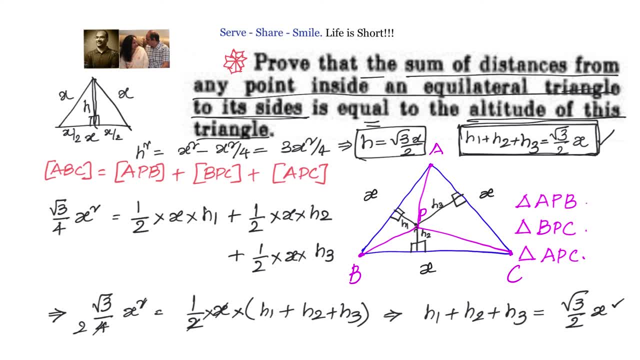 and a line is always the perpendicular distance. So we have dropped the perpendiculars to the corresponding sides. Now we divided ABC into three triangles. Since we know the altitudes, we also know the side. So half into base, into height, We can easily find out the area of. 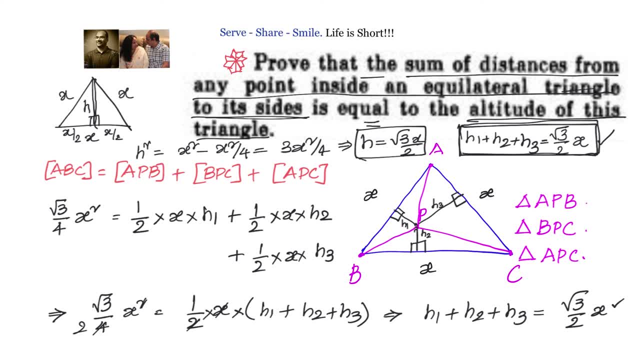 triangle: APB, BPC, ABC. But now these three will add up to area of ABC, which we already know. that root 3 by 4 into x square. Now simplify: We are able to prove that sum of the distances from P to AB, BC and AC is equal to altitude of.